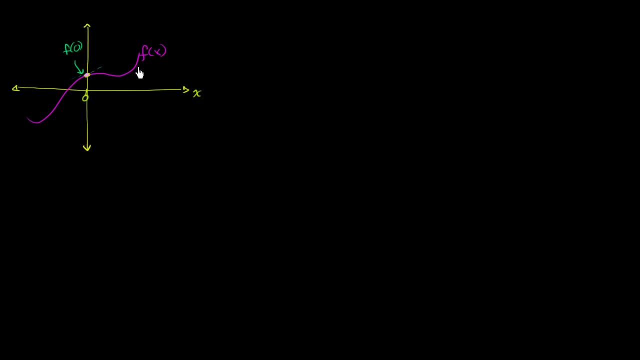 I've drawn an arbitrary function here And what we're going to try to do is approximate this arbitrary function. We don't know what it is, Using a polynomial. we'll keep adding terms to that polynomial, But to do this, we're going to assume that we can evaluate. 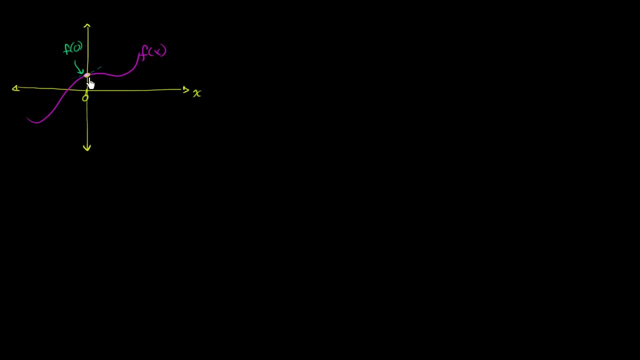 the function at 0, that it gives us some value and that we can keep taking the derivative of the function and evaluating the first, the second and the third derivatives, so on and so forth, at 0 as well. So we're assuming that we know what f of 0 is. 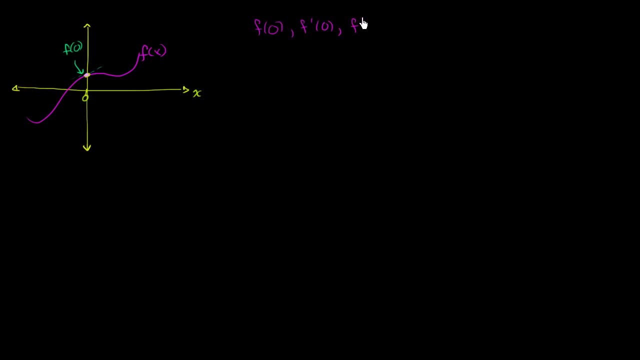 We're assuming that we know what f prime of 0 is. We're assuming that we know the second derivative at 0.. We're assuming that we know the third derivative at 0.. So maybe I'll write it third derivative, I'll just write f prime, prime at 0, so forth and so on. 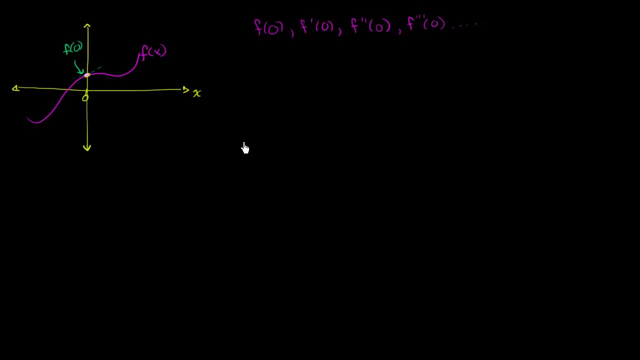 So let's think about how we can approximate this using polynomials of ever-increasing length. So we could have a polynomial of just one term and it would just be a constant term. So this would be a polynomial of degree 0. And if we have a 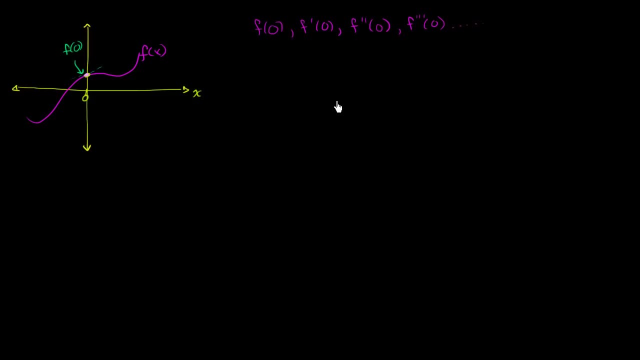 constant term, we could have a polynomial of degree 0. And if we have a constant term we at least might want to make that constant polynomial. it really is just a constant function equal the function at f of 0. So at first maybe we just want p of 0, where p is the 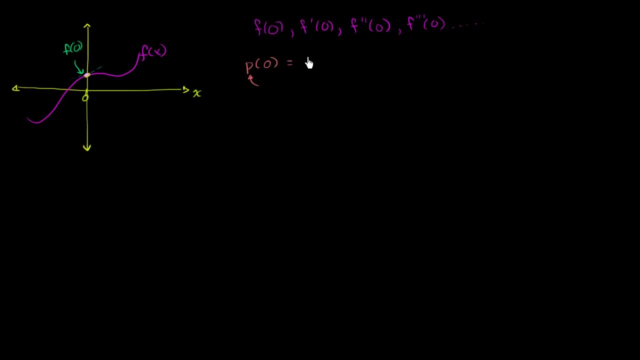 polynomial that we're going to construct, We want p of 0 to be equal to f of 0. So if we want to do that using a polynomial of only one term, of only one constant term, we can just set: p of x is equal. 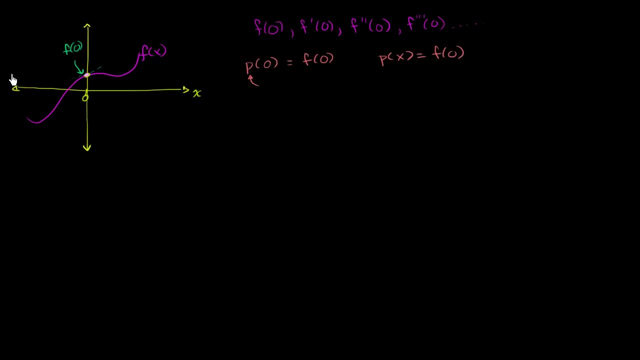 to f of 0. So if I were to graph it, it would look like this: It would just be a horizontal line at f of 0. And you could say, Sal, that's a horrible approximation. It only approximates the function at this point. 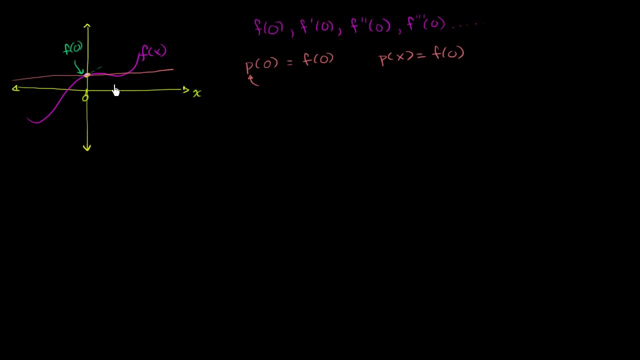 Looks like we got lucky at a couple of other points, but it's really bad everywhere else And I would tell you, well, try to do any better using a horizontal line. At least we got it right at f of 0.. So this is about as good as we can do with just a constant. 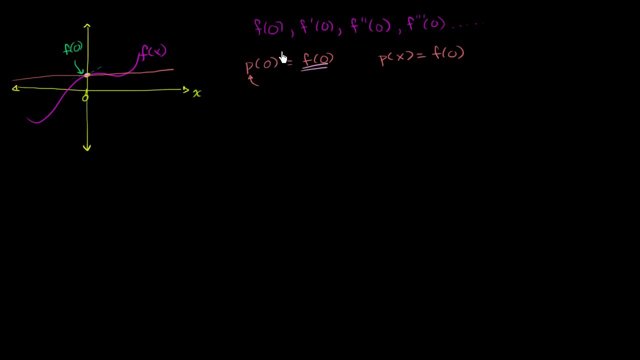 And even though I just want to remind you, this might not be, this might not look like a constant, but we're assuming that, given the function, we can evaluate it at 0, and that'll just give us a number. So, whatever number that was, we would put it right over here. 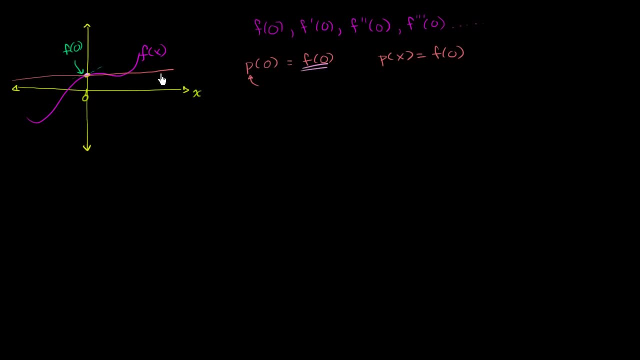 and we'd say p of x is equal to that number And it would just be a horizontal line right there at f of 0. But that obviously is not so great. So let's add some more constraints Beyond the fact that we want p of 0 to be equal to f of 0,. 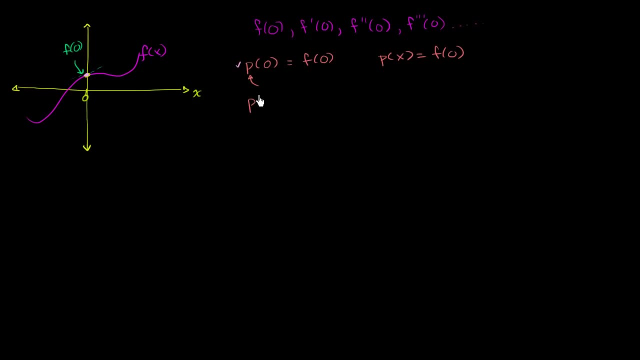 let's say that we also want p prime at 0 to be the same thing as f prime at 0.. Let me do this in a new color. So we also want in the new color. we also want- that's not a new color. we also want p prime. 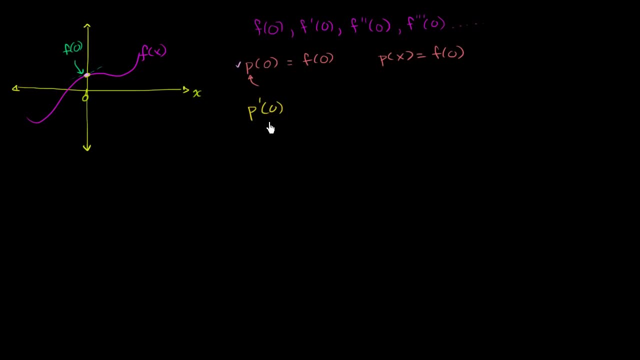 we want the first derivative of our polynomial, when evaluated at 0, to be the same thing as the first derivative of the function when evaluated at 0. And we don't want to lose this right over here. So what if we set p of x as being? 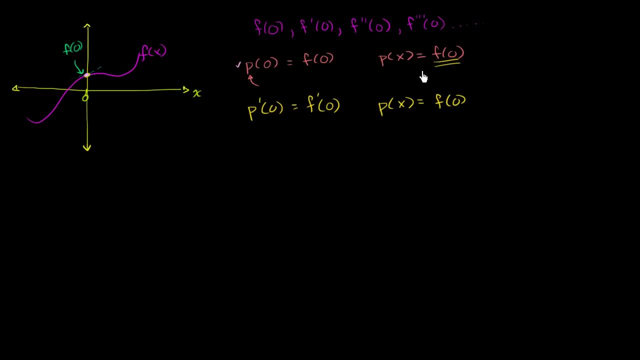 equal to f of 0?. So we're taking our old p of x, but now we're going to add another term so that the derivatives match up Plus f prime of 0 times x. So let's think about this a little bit. 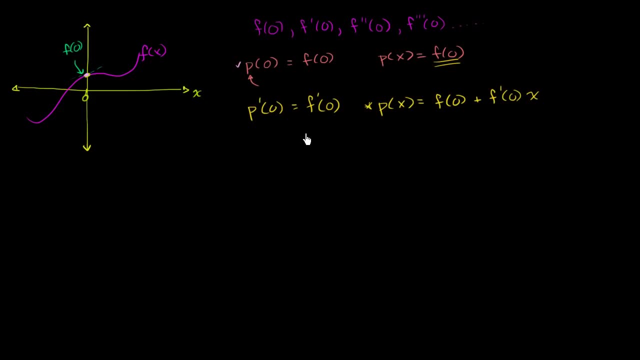 If we use this as our new polynomial, what happens? What is p of 0?? p of 0 is going to be equal to. you're going to have f of 0 plus whatever. this f prime of 0 is times 0.. 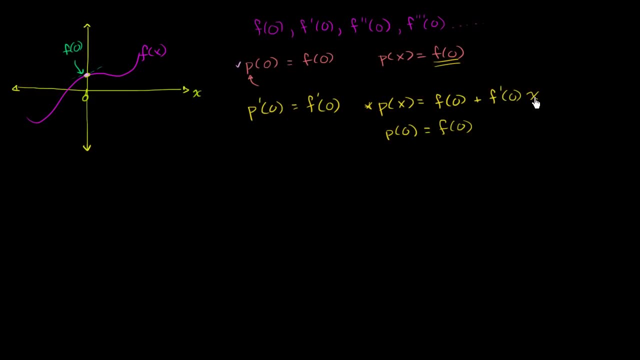 OK, OK, Right. If you put a 0 in for x, this term's just going to be 0. So you're going to be left with: p of 0 is equal to f of 0. That's cool. That's just as good as our first version. 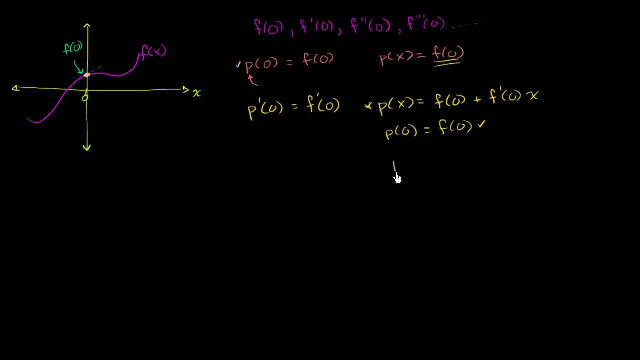 Now what's the derivative over here? So the derivative is p. prime of x is equal. to take the derivative of this: this is just a constant, so its derivative is 0.. The derivative of a coefficient times x is just going to be the coefficient. 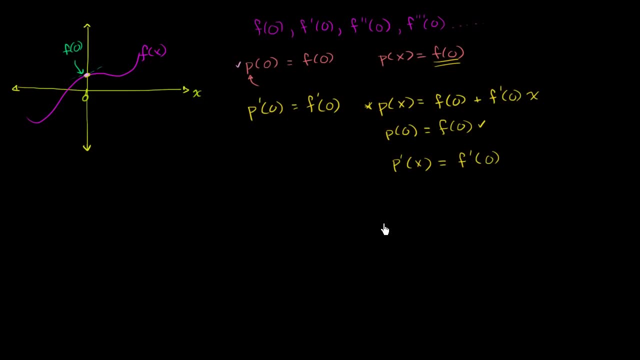 So it's going to be f prime of 0. So if you evaluate it at 0. So p prime of 0, or the derivative of our polynomial evaluated at 0, I know it's a little weird because we're doing all p prime of x, of f, of 0 and all of this. 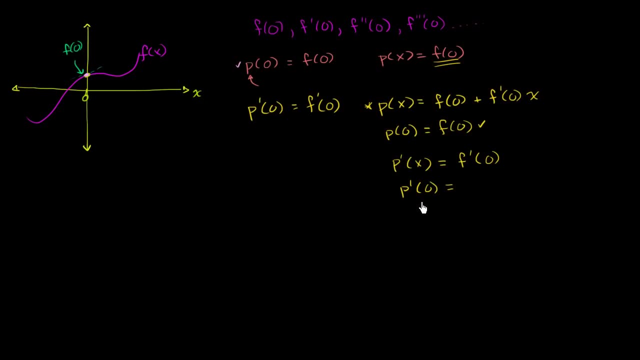 But just remember what's the variable, what's the constant, and hopefully it'll make sense. So this is just obviously going to be f prime of 0. Its derivative is a constant value. This is a constant value. right here We're assuming that we could take the derivative. 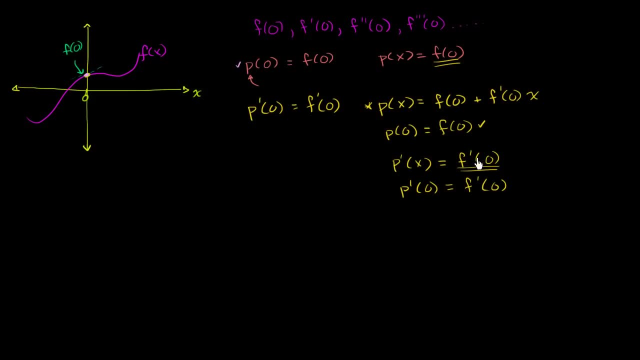 of our function and evaluate that thing at 0 to give a constant value. If p prime of x is equal to this constant value, obviously p prime of x evaluated at 0 is going to be that value. But what's cool about this right here? 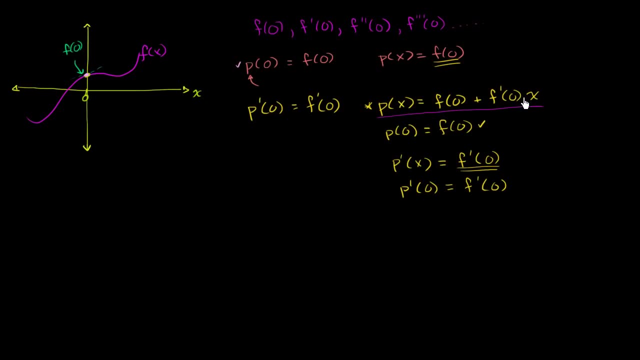 this polynomial that has a 0 degree term and a first degree term is now: this polynomial is equal to our function: at x is equal to 0. And it also has the same first derivative. It also has the same slope: at x is equal to 0.. 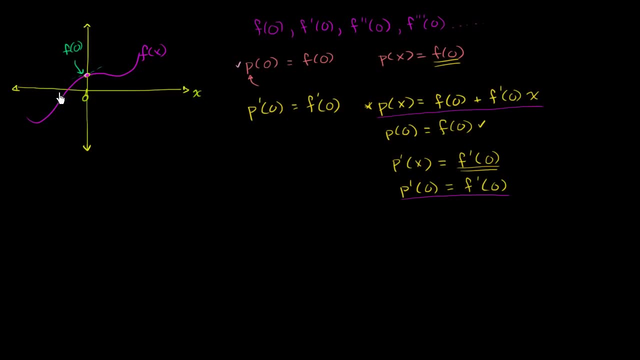 So this thing will look. This new polynomial with two terms is getting a little bit better. It will look something like that. It will essentially have a look like a tangent line at f of 0, at x is equal to 0. So we're doing better, but still not a super good approximation. 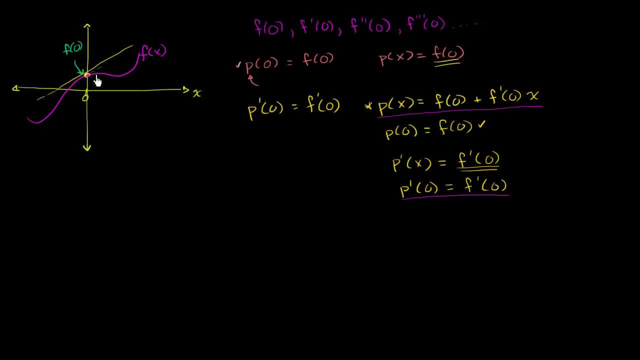 It kind of is going in the same general direction as our function around 0. But maybe we can do better by making sure that they have the same second derivative And to try to have the same second derivative. we can do the same second derivative while still having. 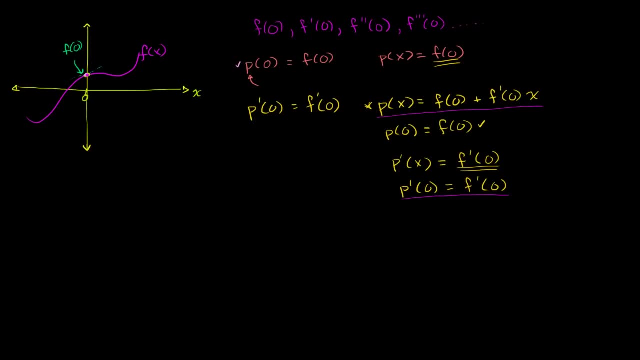 the same first derivative and the same value at 0.. Let's try to do something interesting. Let's define p of x. So let's make it clear. This was our first try. This is our second try right over here, And I'm about to embark on our third try. 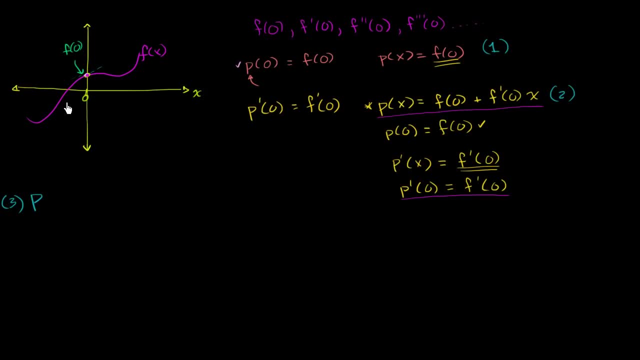 So in our third try, my goal is that the value of my polynomial is the same as the value of the function at 0.. They have the same derivative at 0.. And they also have the same second derivative at 0.. So let's define my polynomial to be equal to. 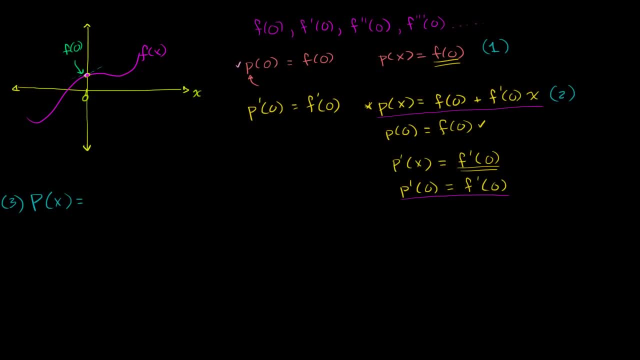 so I'm going to do the first two terms of these guys right over here. So it's going to be f of 0 plus f prime of 0 times x. So exactly what we did here. But now let me add another term. 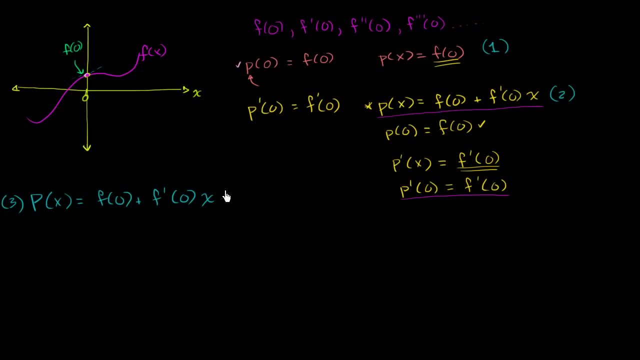 I'll do the other term in a new color, Plus, and I'm going to put a 1 half out here and hopefully it might make sense why I'm about to do this. Plus 1 half times f, the second derivative of our function. 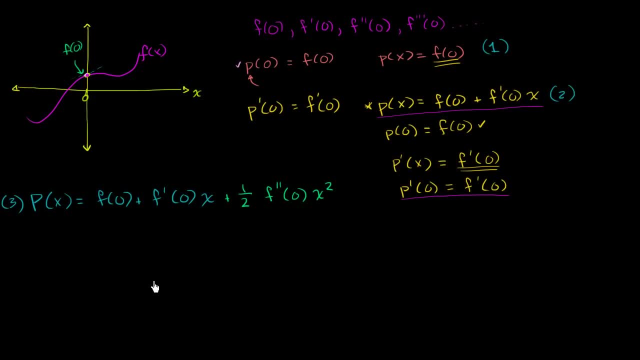 evaluated at 0, x squared, And when we evaluate the derivative of this, I think you'll see why this 1 half is there, Because now let's evaluate this and its derivatives at 0. So if we evaluate p of 0, p of 0 is going to be equal to what? 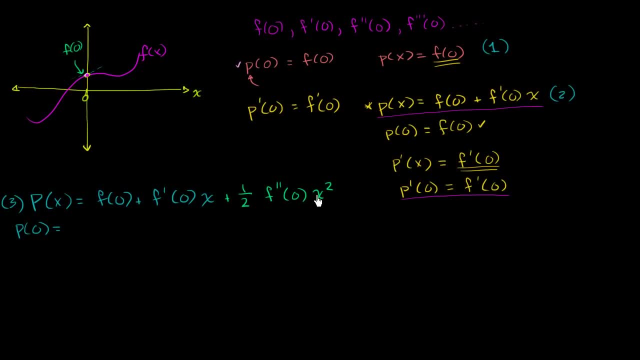 Well, you have this constant term. If you evaluate it at 0, this x and this x squared are both going to be 0. So those terms are going to be 0. They're going to go away. So p of 0 is still equal to f of 0.. 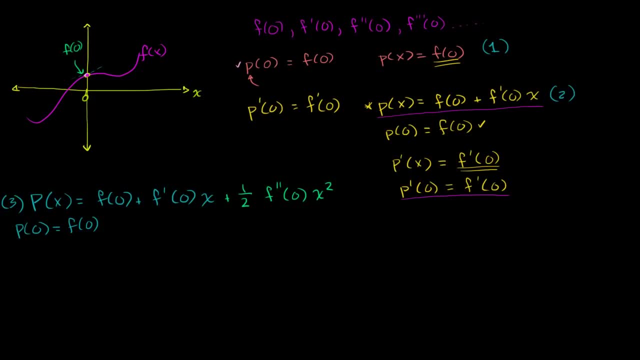 If you take the derivative of p of x. so let me take the derivative right here. I'll do it in yellow. So the derivative of my new p of x is going to be equal to. So this term is going to go away. 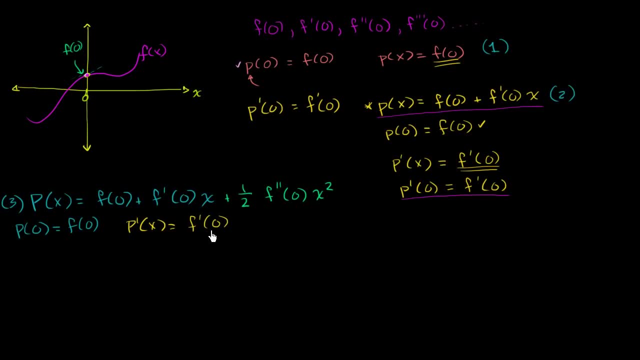 It's a constant term. It's going to be equal to f prime of 0.. That's the coefficient on this Plus this is the power rule right here: 2 times 1 half is just 1 plus f prime prime of 0.. 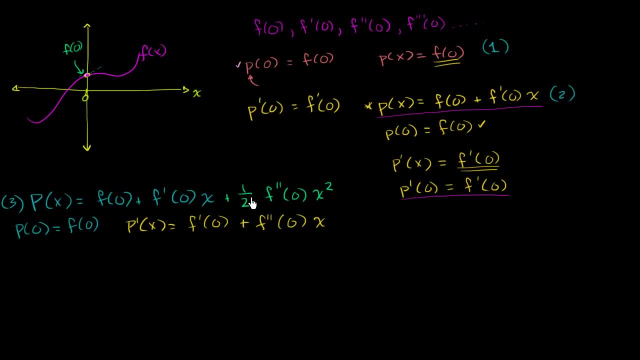 So it's going to be f prime of 0 times x. Take the 2, multiply it times 1 half and decrement that 2 right there, And I think you now have a sense of why we put the 1 half there. 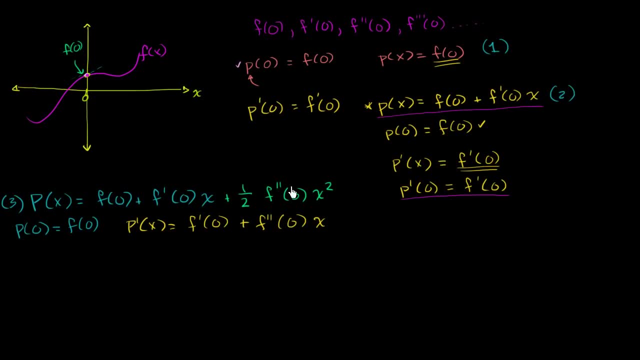 It's kind of counter. It's making it so that we don't end up with a 2 coefficient out front. Now, what is p prime of 0?? So let me write it right here: p prime of 0 is what. 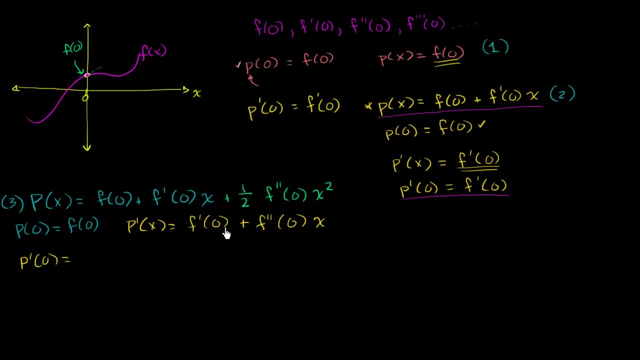 Well, this term right here is just going to be 0. So you're left with this constant value right over here. So it's going to be f prime of 0.. So so far our third generation polynomial has all the properties of the first two. 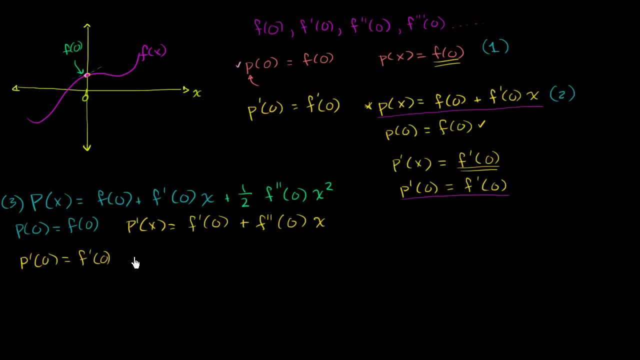 And let's see how it does on its third derivative. So let's see, or I should say the second derivative. So p prime, prime of x is equal to. this is a constant, so its derivative is 0. So you just take the coefficient on the second term. 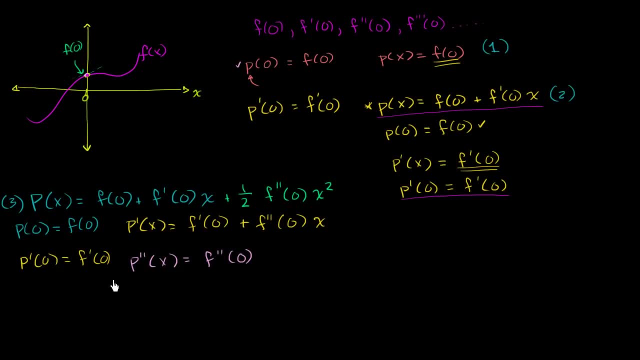 is equal to f prime prime of 0.. So what's the second derivative of p evaluated at 0?? Well, it's just going to be this constant value. It's going to be f prime prime of 0.. So notice, by adding this term now not only. 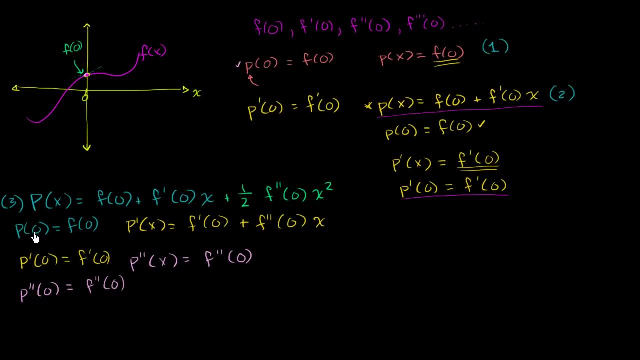 is our polynomial value the same thing as our function value at 0, its derivative at 0 is the same thing as the derivative of the function at 0.. And its second derivative at 0 is the same thing as the second derivative of the function. 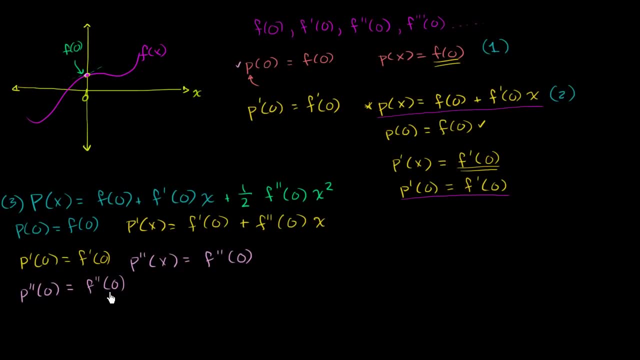 at 0.. So we're getting pretty good at this And you might guess that there's a pattern here. Every term we add. it'll allow us to set up the situation so that the The nth derivative of our approximation at 0. 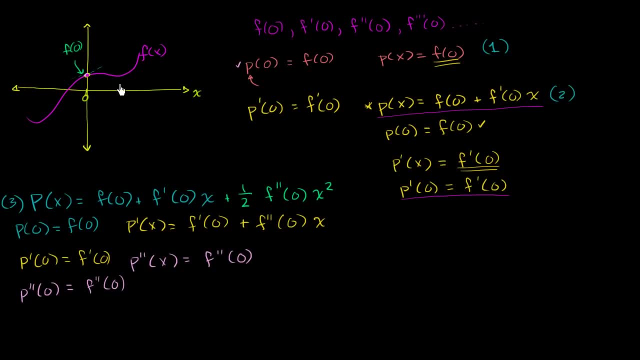 will be the same thing as the nth derivative of our function at 0.. So, in general, if we wanted to keep doing this, if we had a lot of time on our hands and we wanted to just keep adding terms to our polynomial, we could, and let me do this in a new color. 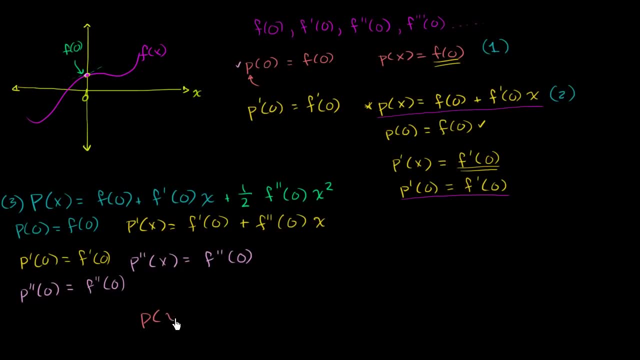 Maybe I'll do it in a color I already used. We could make our polynomial approximation, so the first term, the constant term, will just be f of 0. Then the next term will be f- prime, prime of 0 times x. 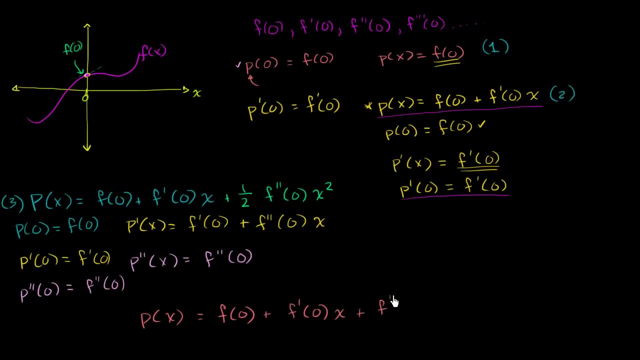 Then the next term will be f prime. prime of 0 times 1, half times x squared. I just rewrote that in a slightly different order. Then the next term- if we want to make their third derivatives the same at 0, would be f prime. 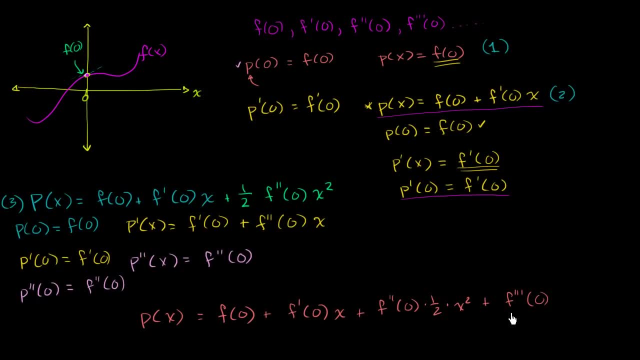 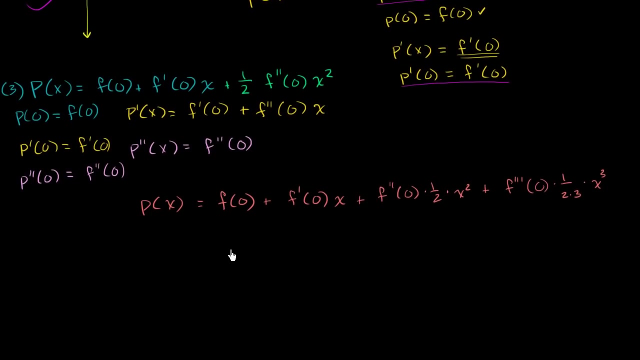 prime, prime of 0, the third derivative of the function at 0, times 1, half times 1, third, So 1 over 2 times 3.. 3 times x to the third, And we can keep going. Maybe you'll start to see a pattern here. 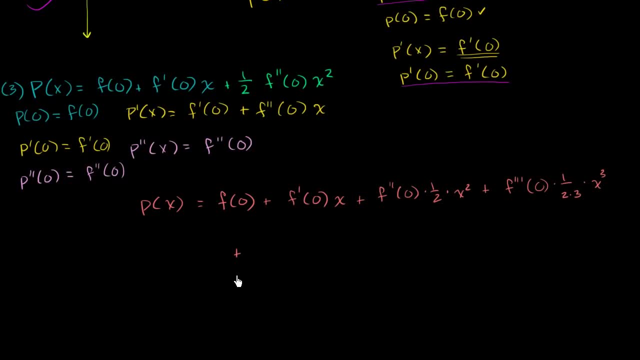 Plus, if we want to make their fourth derivatives at 0 coincide, it would be the fourth derivative of the function. I could put a 4 up there, but this is really emphasizing. It's the fourth derivative at 0 times 1 over. 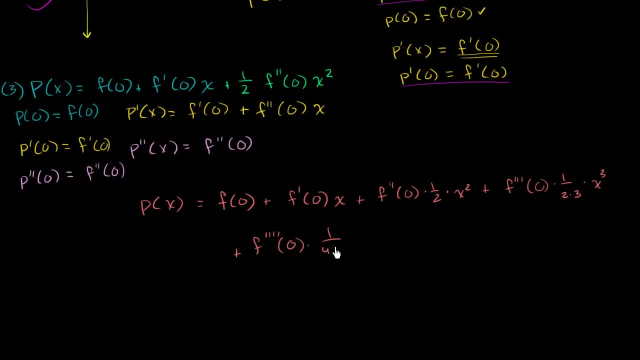 And I'll change the order. Instead of writing it in increasing order, I'll write it as 4 times, 3 times 2 times x 1 to the fourth, And you can verify it for yourself. If we just had this only and if you. 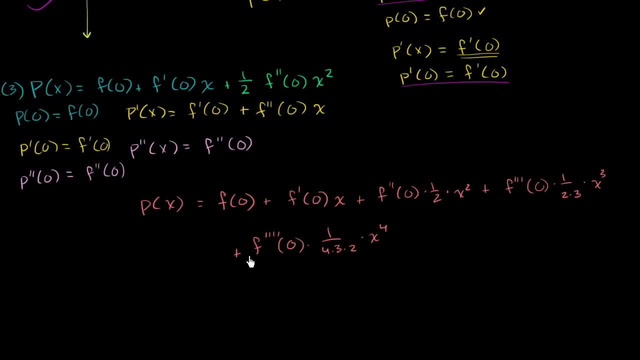 were to take the fourth derivative of this, evaluate it at 0,, it'll be the same thing as the fourth derivative of the function evaluated at 0.. And in general, you can keep adding terms where the nth term will look like this: 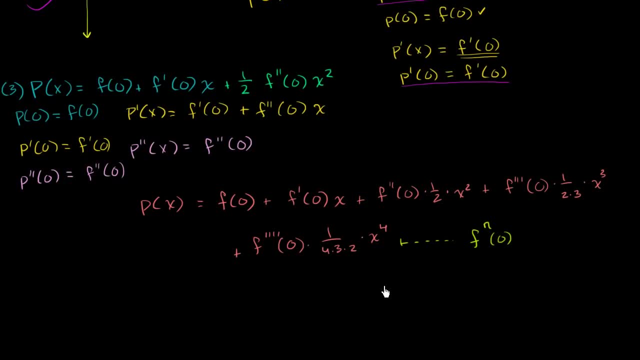 The nth derivative of your function, evaluated at 0, times x to the n over n factorial. Notice This is the same thing as 4 factorial. 4 factorial is equal to 4 times 3 times 2 times 1.. 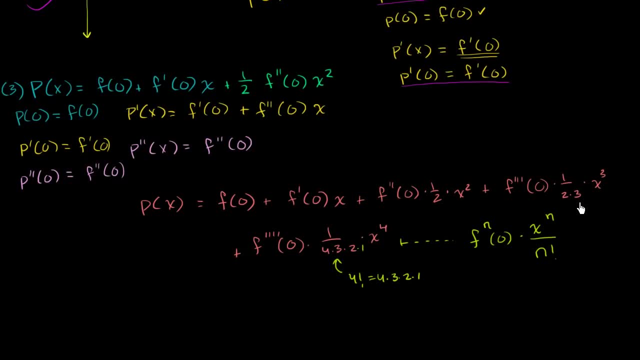 You don't have to write the 1 there, but you could put it there. This right here is the same thing as 3 factorial 3 times 2 times 1.. I didn't put the 1 there. This right here is the same thing as 2 factorial. 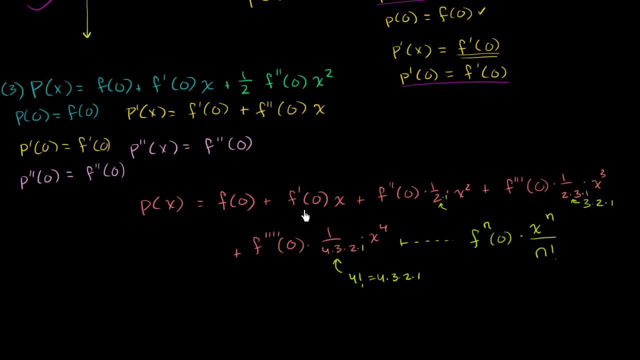 2 times 1.. This is the same thing. We didn't write anything, but you could divide this by 1 factorial, which is the same thing as 1.. And you could divide this by 0 factorial, which also happens to be 1.. 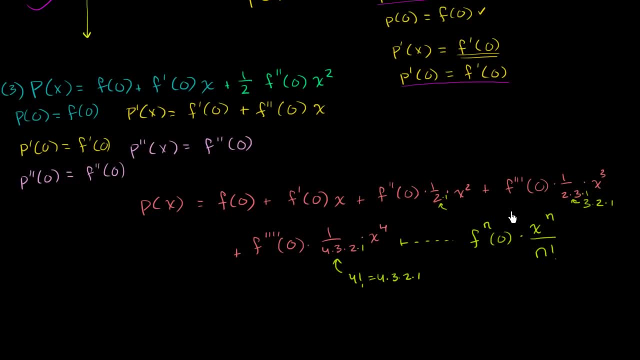 We won't have to study it too much over here. But this general series that I've kind of set up right here is called the Maclaurin series, And you can approximate a polynomial And we'll see at least some pretty powerful results. 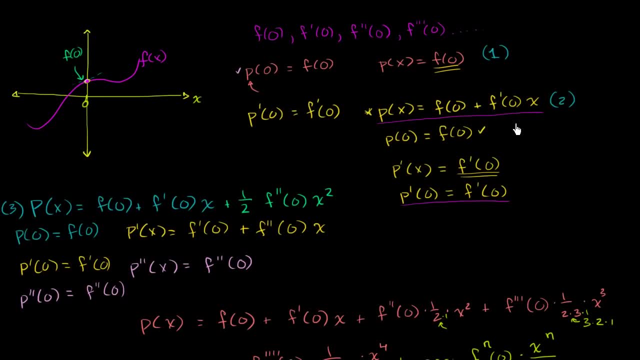 later on. But what happens- and I don't have the computing power in my brain to draw the graph properly- is that when only the function is equal, you get that horizontal line. When you make the function equal at 0, and their first derivative is equal at 0,. 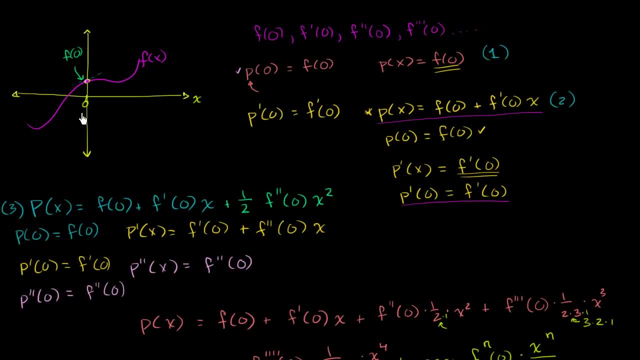 then you have something that looks like the tangent line. When you add another degree, it might approximate the polynomial something like this: When you add another degree, it might look something like that: And as you keep adding more and more degrees, or when you keep adding more and more terms, 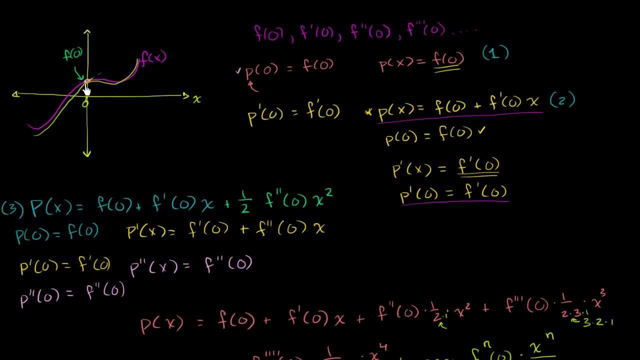 it gets closer and closer around, especially as you get close to x is equal to 0. But in theory, if you add an infinite number of terms, you shouldn't be able to do it. I haven't proven this to you, So that's why I'm saying it's in theory. 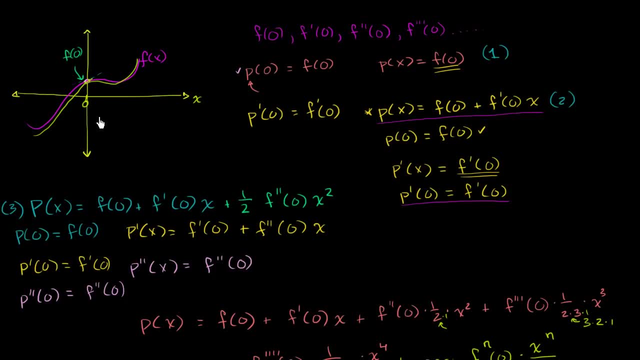 I haven't proved it yet to you, But if you add an infinite number of terms, all of the derivatives should be the same, And then the functions should pretty much look like each other. In the next video I'll do this with some actual functions.